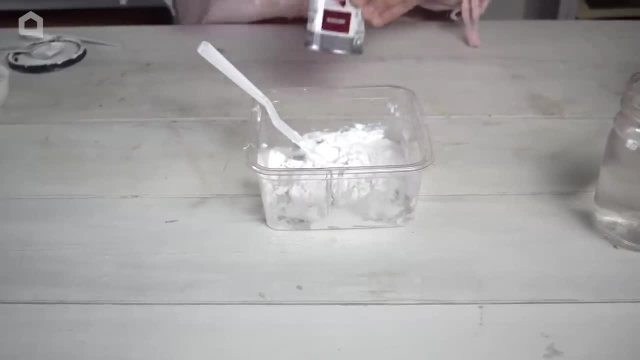 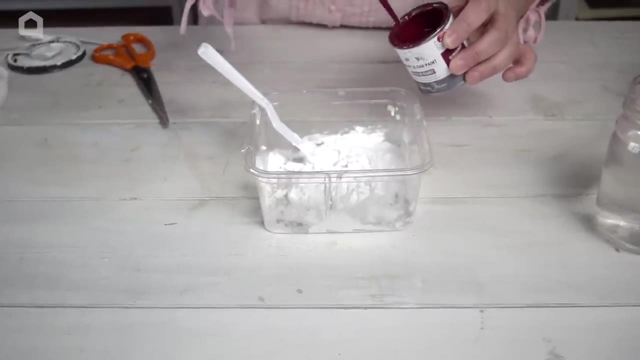 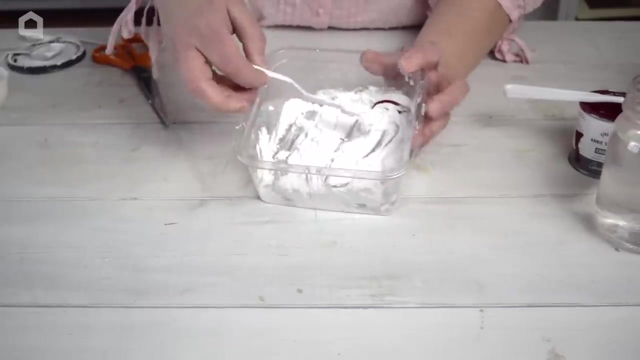 so I'm going to put just a dab of this paint in next, and I'm going to put this in now so that it can be mixed in with my paint. There's a couple of different ways that you can do this, but I like to add it at this point of the mixing process, but you can also do this after you've got your art piece. 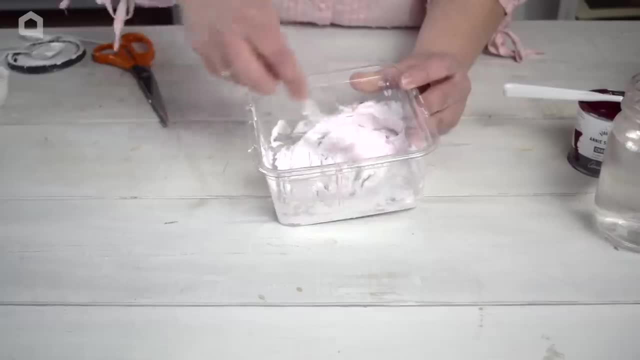 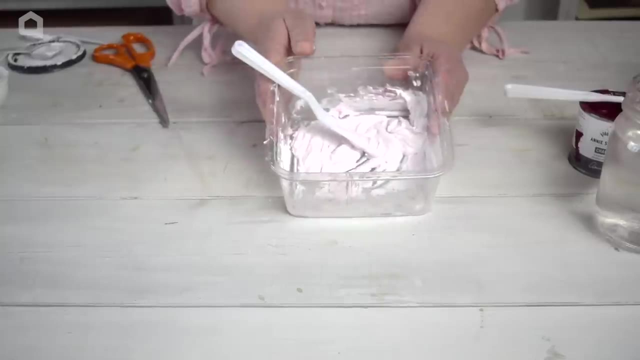 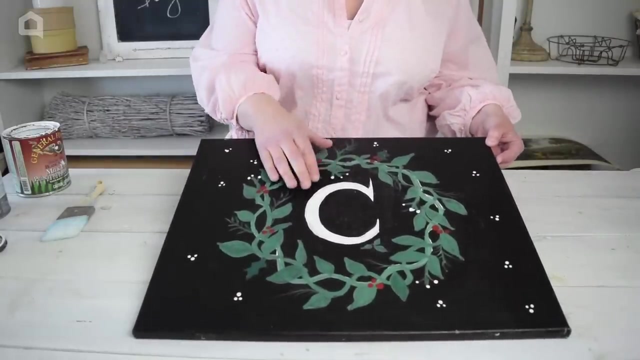 made and then paint it. Okay, there we go. so my paint, my 3D paint here is ready to go, and I'm going to grab my canvas and show you what we're going to do. To get started on our project, I'm going to reuse an old canvas that I picked up at the thrift store for two dollars. I really like. 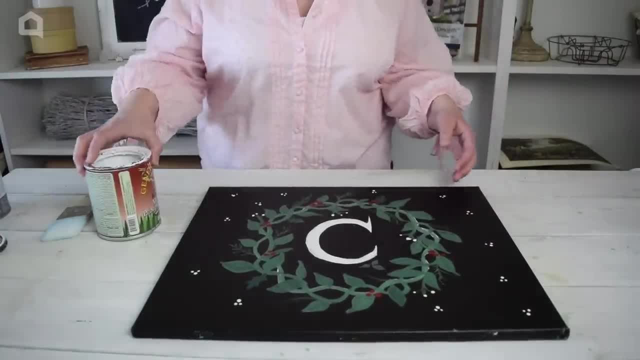 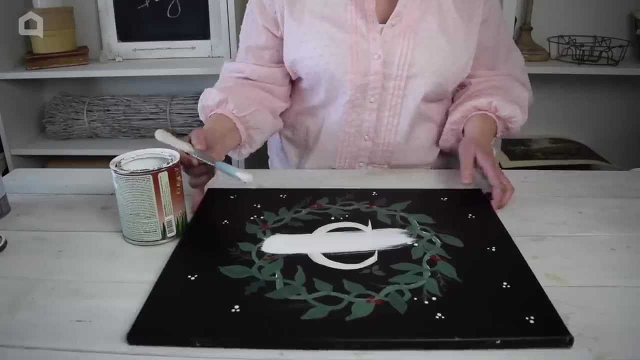 reusing old canvases instead of using new ones. So I'm going to take my 3D paint and I'm going to buy a new one so that we can reuse something that's already out there. So to prep my canvas for this art project, all I need to do is take some white paint and I'm just going to cover this up. 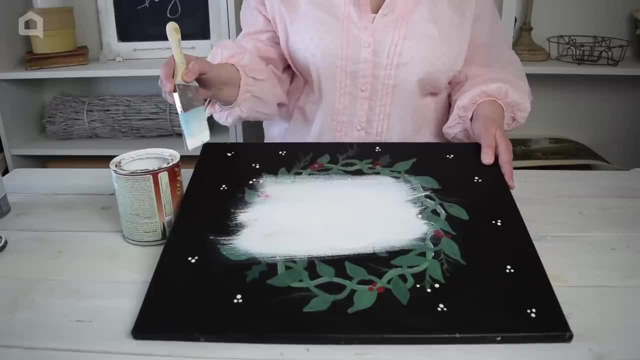 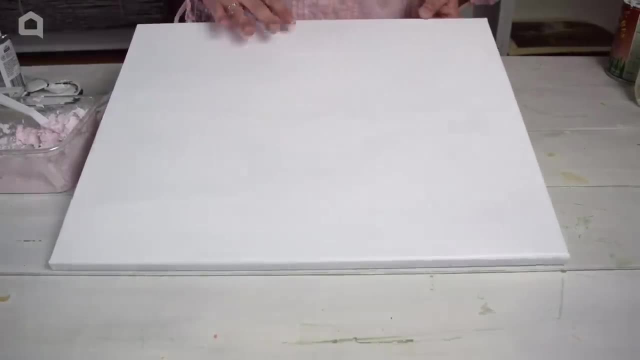 It'll likely take two coats to cover up the paint that's already on here. My canvas is all prepped and ready to go now, so that the black canvas that I found for a couple dollars is all nice and white and it's ready to go, and I also have my paint ready to go and what I want to do is create a. 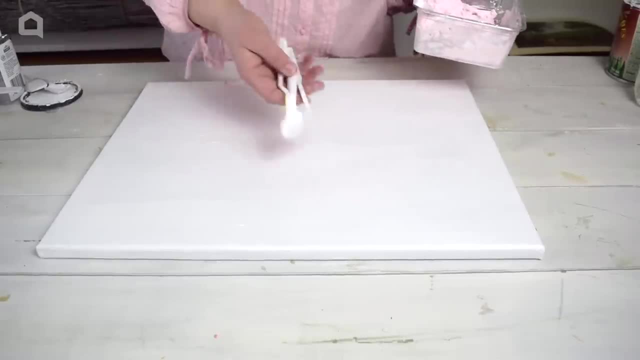 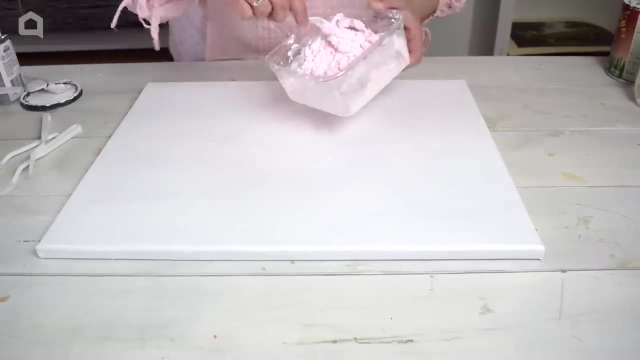 beautiful big spring flower here. I'm going to take my 3D paint and I'm going to put this in here, So to make your petals you can use any sort of little spatula or spoon, however you like to make them, and we want to take our paint and I'm going to kind of center my flower on this side. so 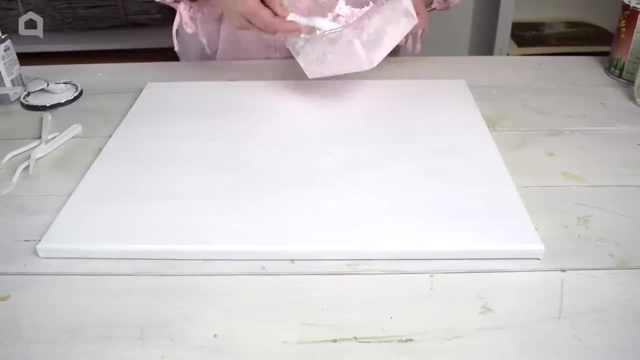 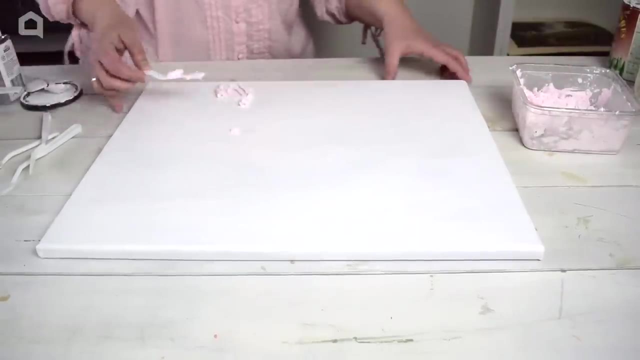 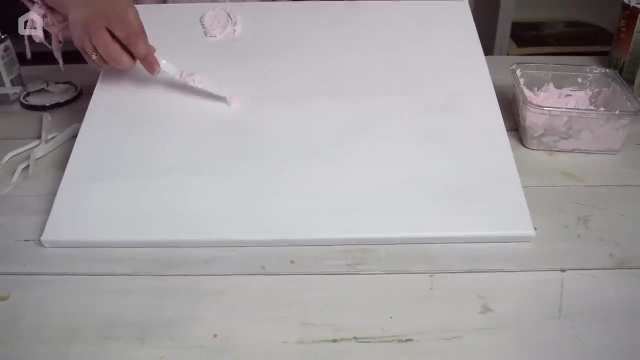 I just want to center it a bit off and I'm going to start using this paint to make really chunky petals. So I'm just going to spread it around like this and let me hold this up here. I am going to center here and I can kind of put that there to mark my center, although it will be a different. 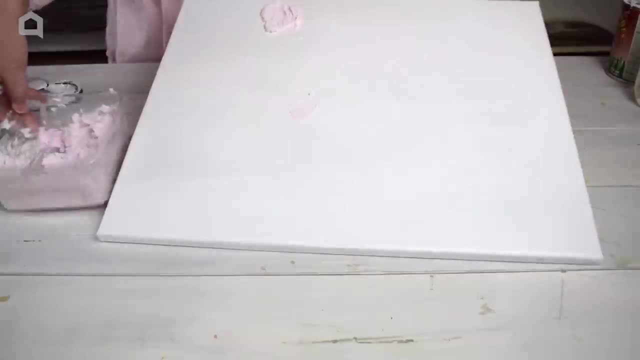 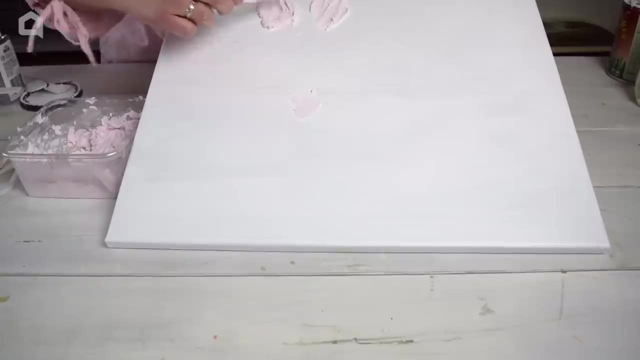 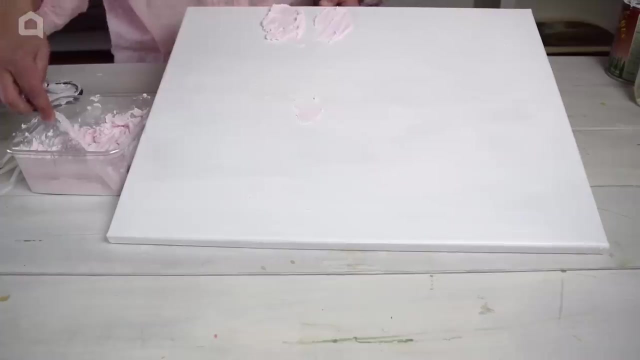 color later. So I'm going to keep taking my paint here and I'm going to start with that outer ring of petals for my flower and I just want to goop this on however you'd like. I want to make my petals really nice and big and almost like they're coming off the edge of my canvas here. 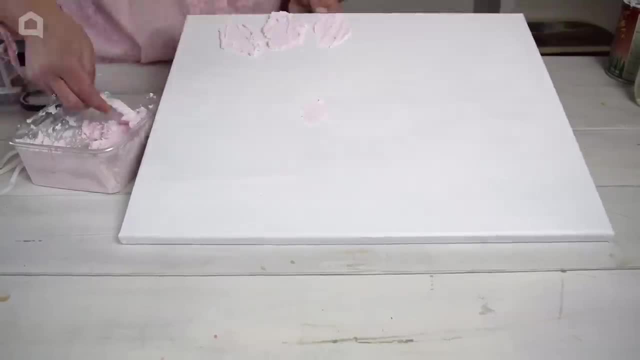 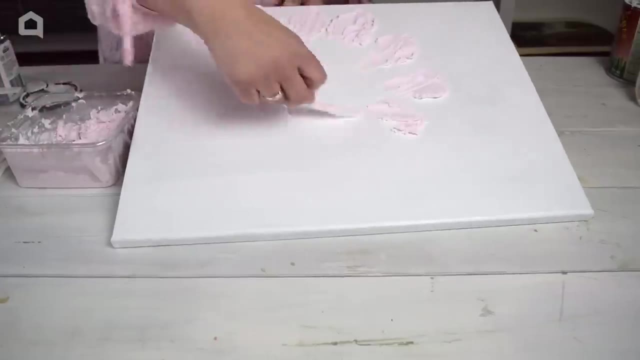 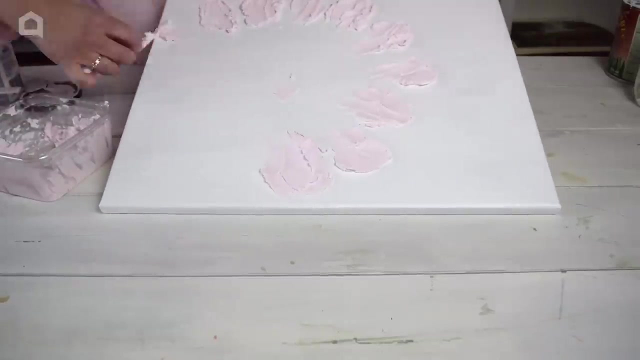 working towards that center, Starting with the lightest color on the outside here, and all I'm going to do is keep working around with these nice. these are going to be the outer, outer edge of the petals and you want to leave it nice and chunky on your canvas. Don't worry about smoothing it out, You'll have lots of time to work. 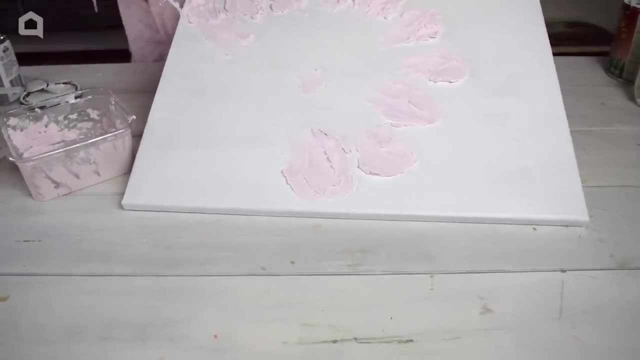 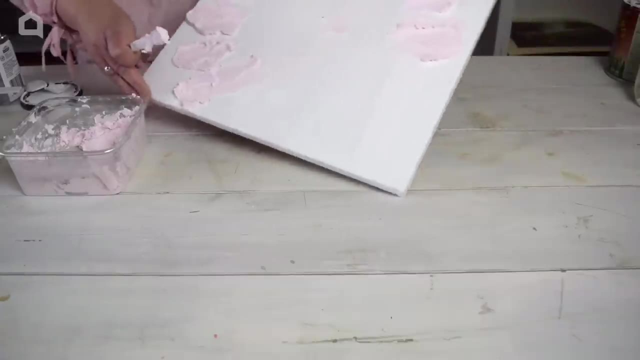 with this, because it does take a bit of time to dry. so don't worry about doing all of your details right away. You'll have lots of time to play with this. I'm just going to turn my canvas here so I can work this direction. 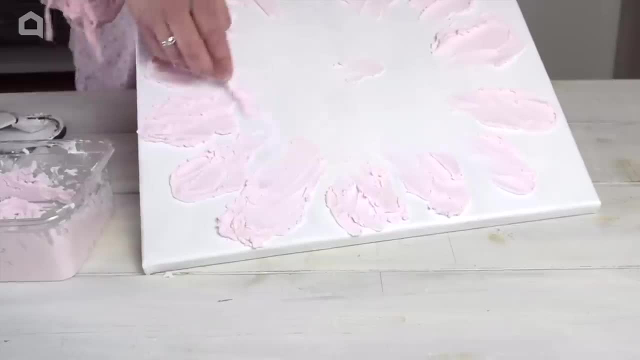 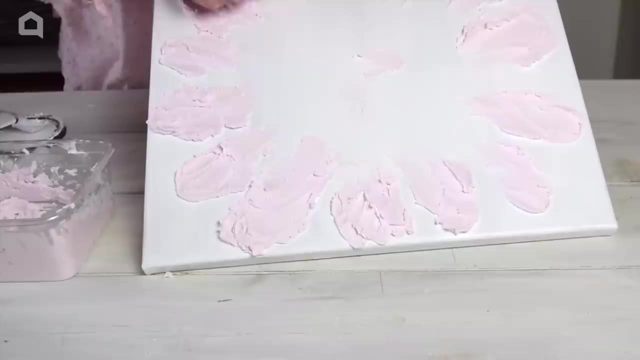 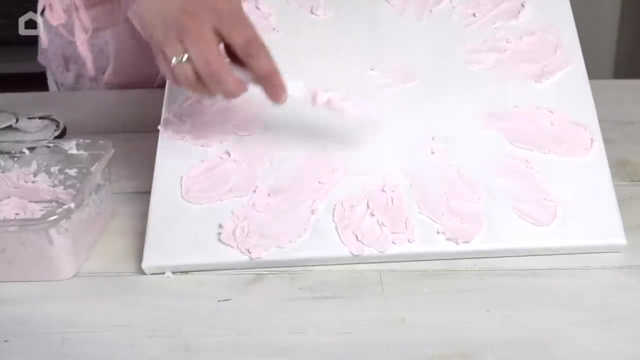 and I'm just going to smooth out the bottoms here so that I can add another layer of petals. I'm going to make some more paint and then I'm going to add a closer layer of petals and as I work my way in, I'm going to get darker and darker. I've gone ahead and 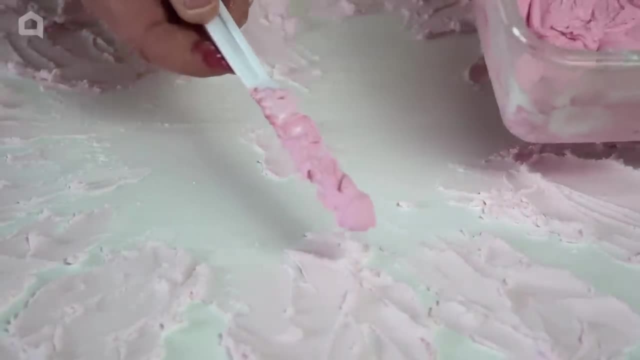 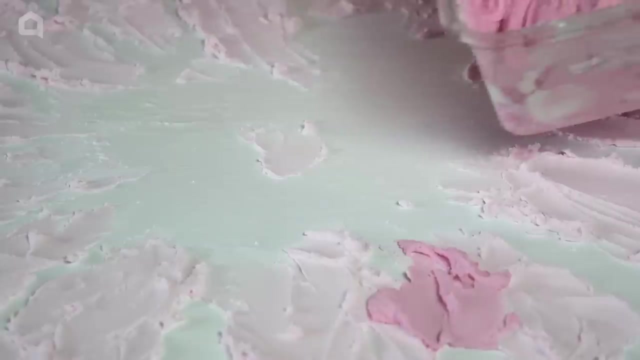 mixed up another batch of paint, and this time I made it just a shade darker than what I did originally. now I'm going to start putting on another layer of petals, and I want these petals to be in between the first ones, and I'm just going to keep pulling it. 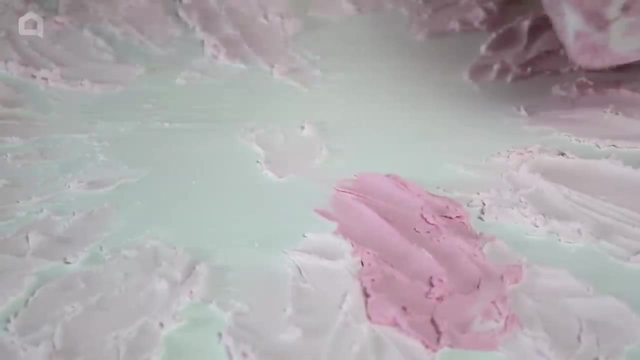 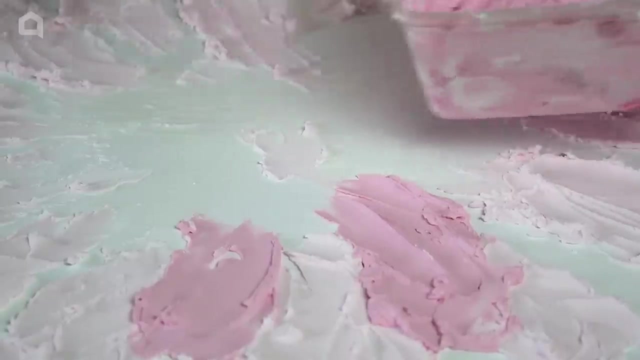 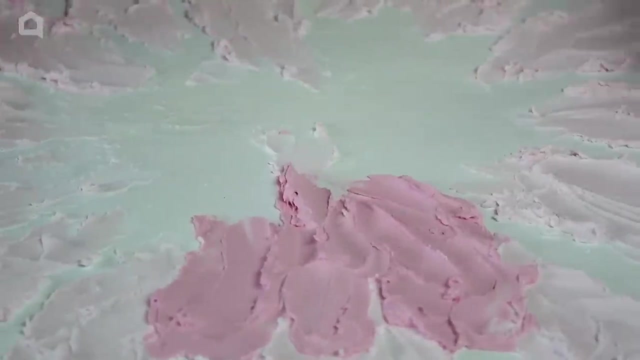 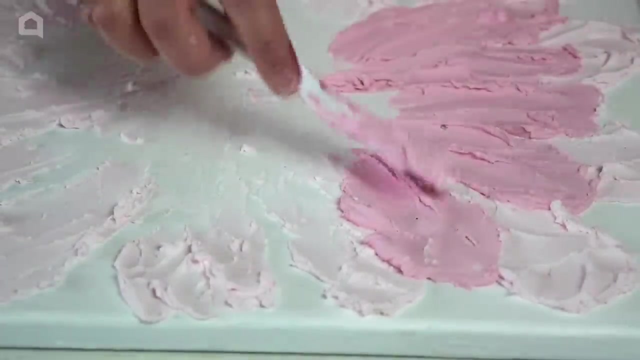 further back towards the center of my flower, and I like doing this while the other layer of petals is still wet, so that I can mold it and smooth it out if I need to, and you just want to keep putting this layer in between the first ones now that I've added a little bit more of the colored paint to my mixture. 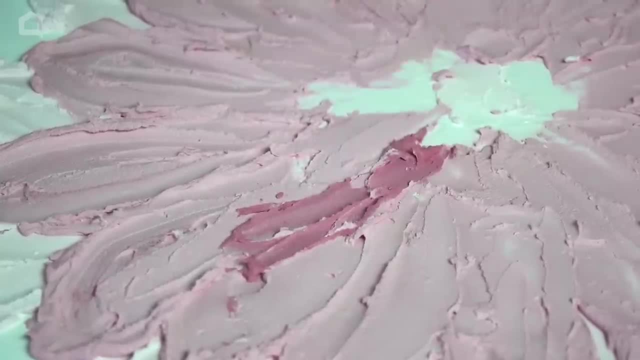 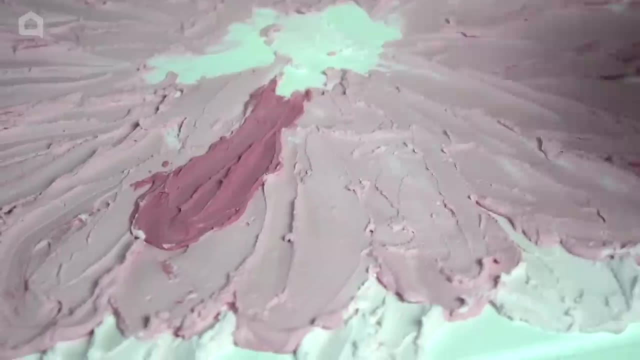 here I'm ready to put on my final layer of petals before I do the center. so I'm just gonna make some small petals in between and again, I have not waited for this to dry for a couple of days and I'm just going to apply my first one here. 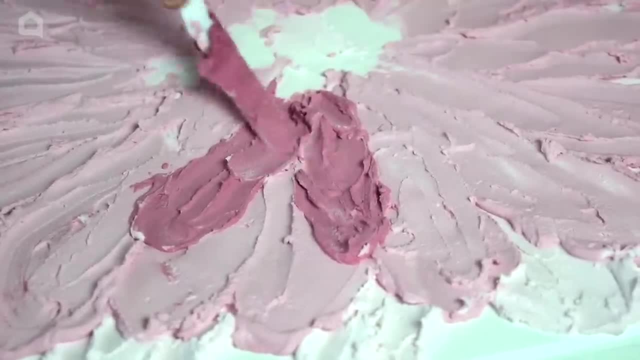 and then I'm just going to put a little bit more of the colored paint on, and then I'm just going to put a little bit more of the colored paint on and this to dry. I like to do this when it's still the other layers are still wet, so 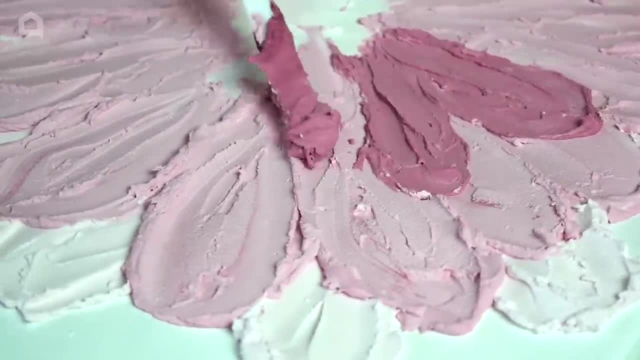 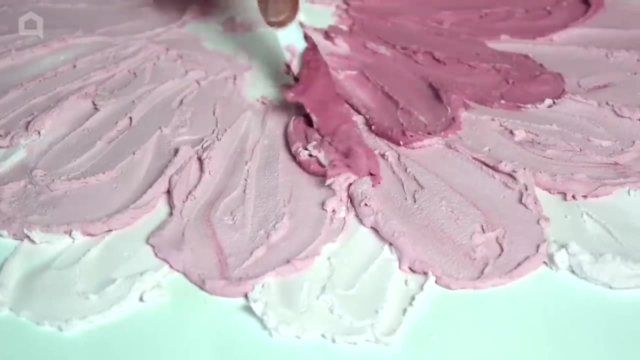 I'm just gonna form some little petals coming into the center here, and you can make as many or as few petals as you want. you just want this to be a nice full flower. once the inner circle is done like this, I'm going to let it start.